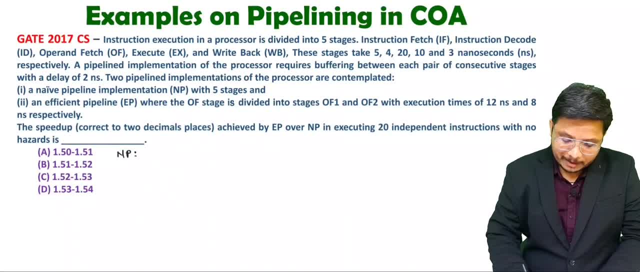 So let me notround down things. See, first I will be considering non-efficient pipeline nd. in that, what are the delays? Let me mention that five, Four to twenty, ten and three, right, And that is that in terms of nanosecond. and let me note down efficient pipeline over here. So, in efficient pipeline, what are the delays? So, third stage that we are changing right l. 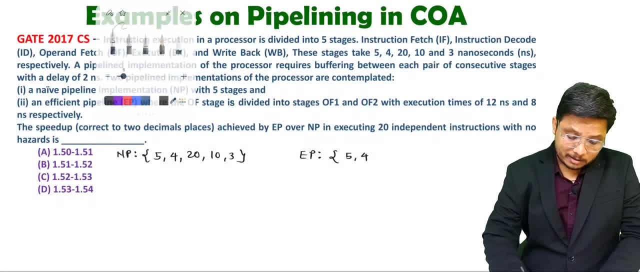 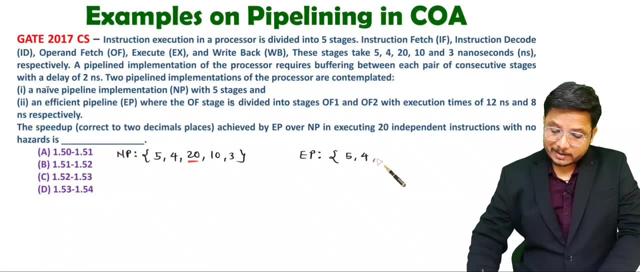 So first two stages is, as it is, five and four, But here third stage. you see, third stage, that is operand fetch that is bisected into 2, 12 and 8 nanosecond. so here i am mentioning that 12 and 8 nanosecond. then again things are same, so 10 and 3, right. so by this red color you 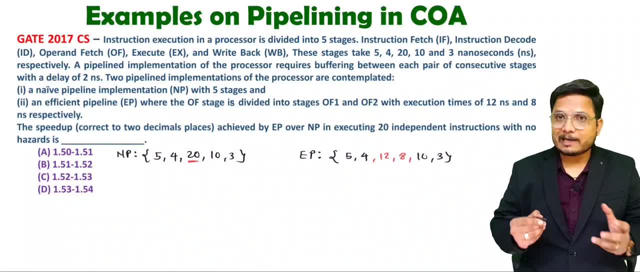 see modification that is done, and that is what efficient modification that is given. and based on that, what is the speed up? that is equation. so here, first of all, you will have to identify how many stages are there over here. so let us say k1, that is 5 over here, and over here, how many? 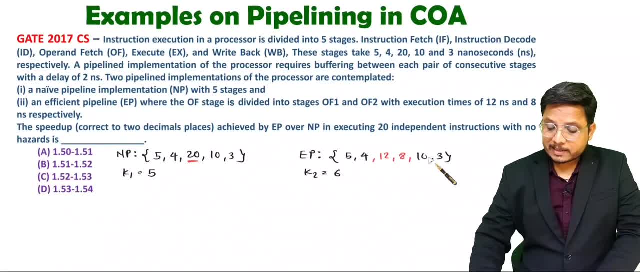 stages are there. let us say k2. so that is 6 over here. 6 stages are there over here. what is the cycle time of each stage? so cycle time of each stage: that will be the maximum time of these stages. so maximum is 20. so cycle time: that will be 20 nanosecond over here with non-efficient. 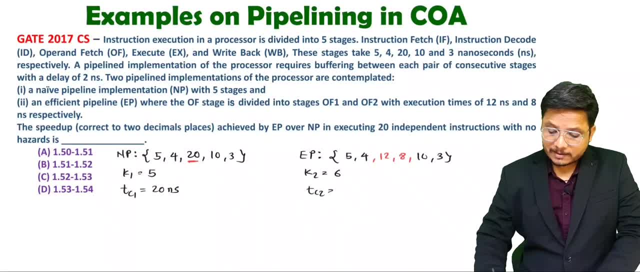 pipeline, but with efficient pipeline. cycle time is you, highest is 12, so here, 12 over here. but, my dear students, you see delay of 2 nanosecond that is given in between consecutive pair, so as delay of 2 nanosecond that is given in consecutive pair. 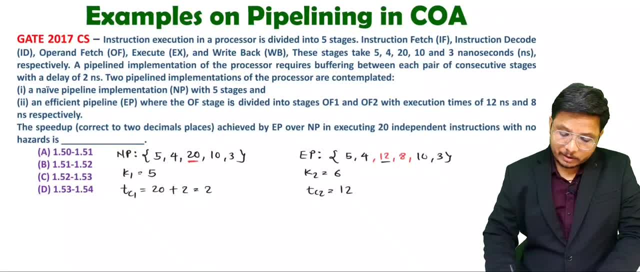 along with this 20, we need to add 2 that is 22 nanosecond, and along with this 12, we need to add 2 that will be making it to 14 nanosecond. i have seen students are making this small mistake, so remember, as if delay is given, then highest delay of stage plus you'll have to add delay of. 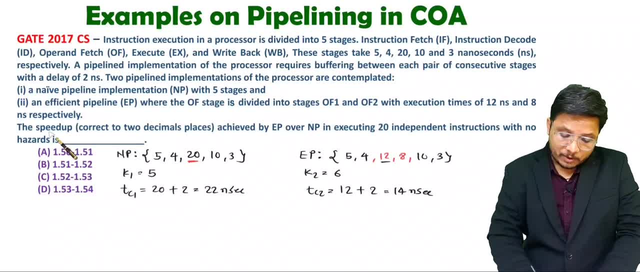 that buffer right now, as if you want to calculate speed up, then calculation is very simple. speed up is time pdr required for non-efficient pipeline divided by time pdr required for efficient pipeline. so what is the time pdr which is there with non-efficient pipeline with non-efficient 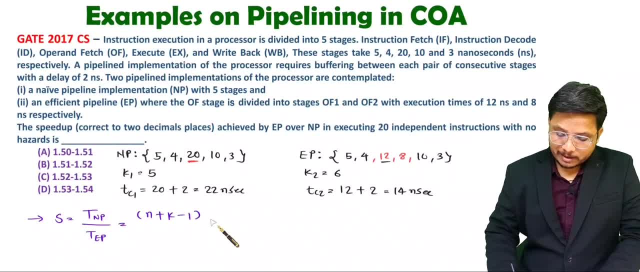 pipeline n plus k minus 1 into tc1- right, and here instead of k i'm writing k1- and with efficient pipeline n plus k2 minus 1 into tc2. let us substitute the values. so how many instructions? 20 instructions are there, plus k1. 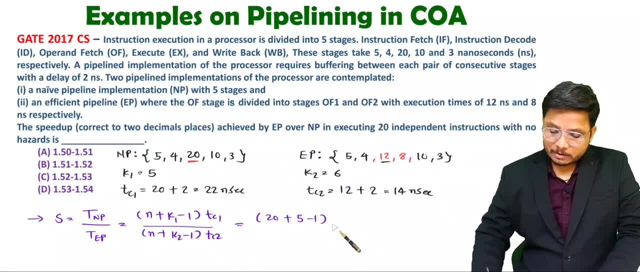 that is pi minus 1 into. delay is 22 over here. with cycle time divided by number of instruction, that is 20 plus stages, are 6 minus 1 into this time, pdr is 14 nanosecond right, and here instead of k i'm writing k1. and with efficient pipeline, n plus k2 minus 1 into. 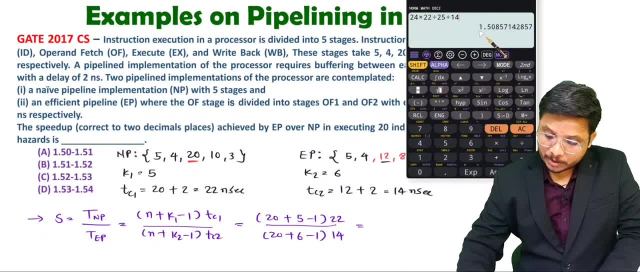 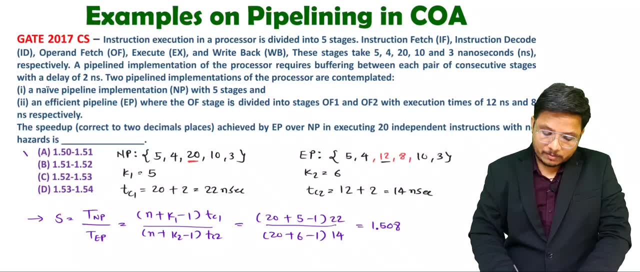 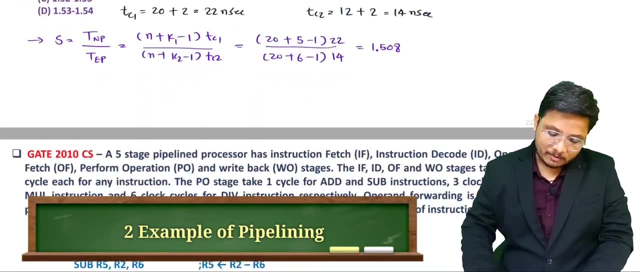 tc2. let us solve this in calculator. so answer is 1.508. so if you observe our options, 1.502, 1.51. so option a is correct, right. so that is how we can easily solve questions. let us have second question over here. so if you observe second question in that, a five stage pipelined processor. 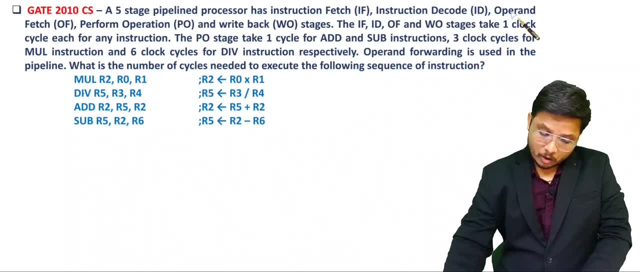 has instruction, fetch instruction, decode operand fetch, perform operation and write back stages. in short form, it is written: i f, i, d, o, f w o right. this four stages takes one clock cycles. that is written and this one stage, that is perform operation, means it is there. with respect to alu. 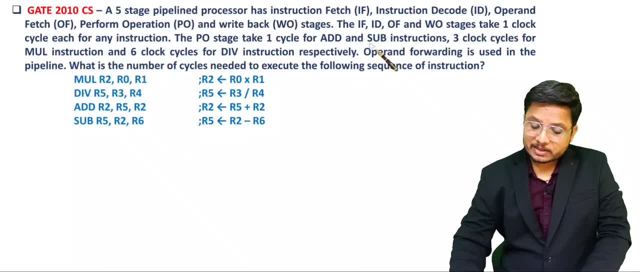 that will be taking one cycle for add and subtraction instruction and three clock cycles for multiplication and six clock cycles for division respectively. operand forwarding is used. see, this is very essential. operand forwarding is used right in pipeline. what is the number of cycles needed to execute the following sequence of instruction? 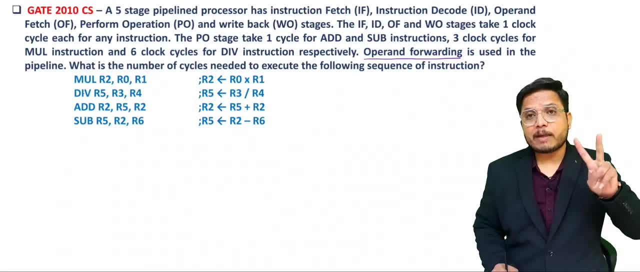 so here, my dear students, i'll explain you this solution by two different ways. one is normal calculation and second is based on your simple logic. see, operand forwarding is given, as if operand forwarding is given, then you don't need to see operands in instructions, like you see. here operands are given, so all these operands that we do don't need to see even why. the reason is we have no go to movie. Extension思ع jión yóng5 yóng 5 yóng1 N? breea0 šwîājsli RPG. oiz새âm äp ateúpand iständi yÉĦ productivity, lw 155 다음. 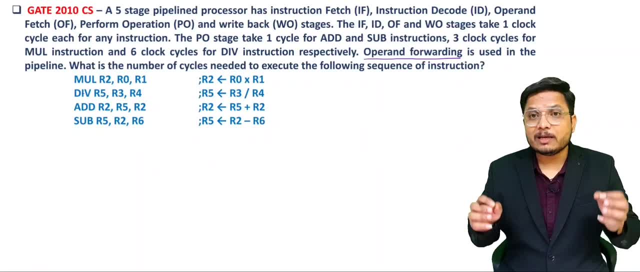 you need to see operands in instruction, like you see here operands argument. so all these operands that we listens to, to monitor them, you should perform instead of changing operation function you have knowledge is operand forwarding will solve issues of data dependency. in this video itself i'll explain you. 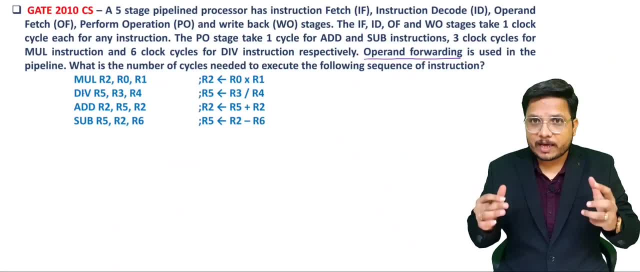 same question, along with without operand forwarding. but let us try to understand this question first with operand forwarding, right? so here see, we are having five stages in multiplication. we need to have three clock cycle in perform operation, right, let me mention that three perform operation over here and with division we need to have six. with addition and subtraction we need to have one. 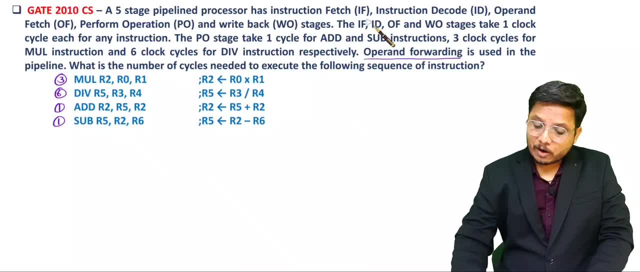 clock cycles only four, perform operation right, otherwise all the stages is having only one cycle only. so, first of all, what i'll do is i'll explain you this explanation with respect to instruction execution. so let us say: this is i1, this is i2, this is i3 and this is i4. so when you execute i1, 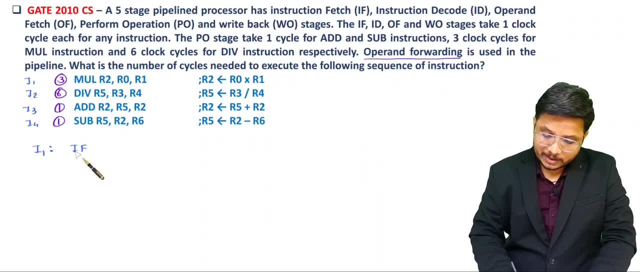 what you will be doing. first you will be performing instruction fetch, then instruction decode, then operand fetch, then perform operation. so you see, multiplication is having how many perform operation three. so po, po, po, three times. i'm writing it, then we are having: write back means wo? right now, my dear students, let us execute second instruction. so instruction fetch. 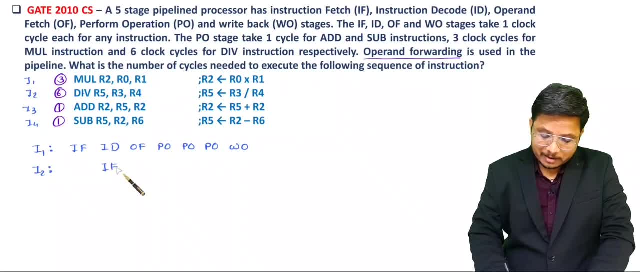 that will happen over here in pipelining, then instruction decode will happen, then operand fetch that will happen, but perform operation. that is not possible here. why? the reason is, if you observe, alu is busy in executing first instruction, so here there will be stalling of pipeline because of. 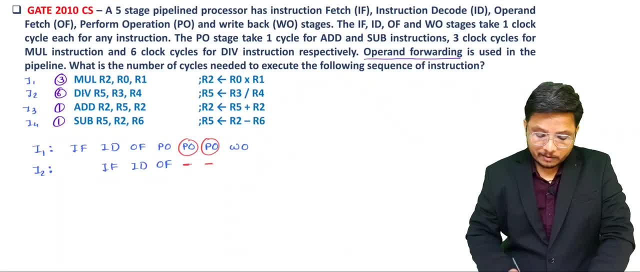 structural hazard, right, so here you will have to wait with second instruction. why? the reason is perform operation. that cannot be done over here, as i1 is doing it right now. my dear students, perform operation will start over here. you see, write back is happening here, so So perform operation can be done here. 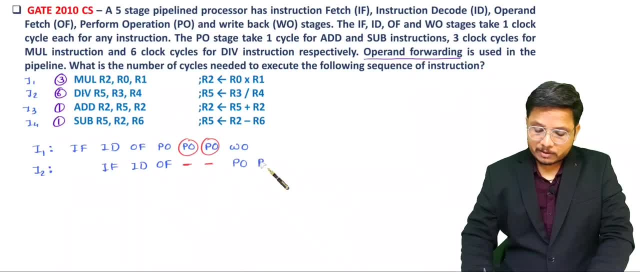 With division. how many perform operations? are there Six, So PO that I need to write six times, right, As it needs six cycles to execute that. So six times PO is written. After that write back is happening right Now if you observe I3 execution. 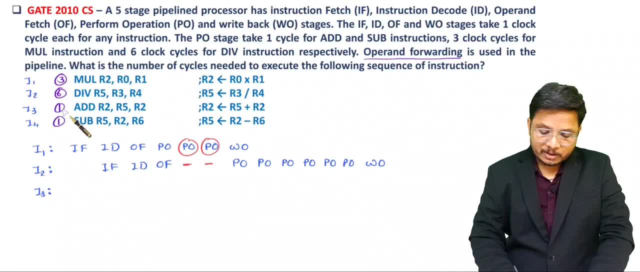 So in that addition is there In that with perform operation only one cycle requires. So IEF means instruction fetch will happen here, Instruction decode will happen here, Operand fetch will happen here. But you see here perform operation, that is there with I1, right. 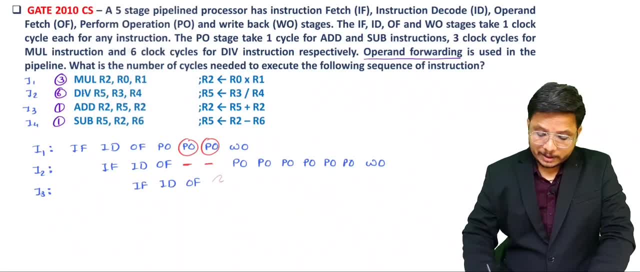 So CPU is busy. So all you need to have is you need to wait for that ALU to be free. So here it is busy, Here it is busy, Here it is busy right Now, you see, here onwards, that ALU is free. 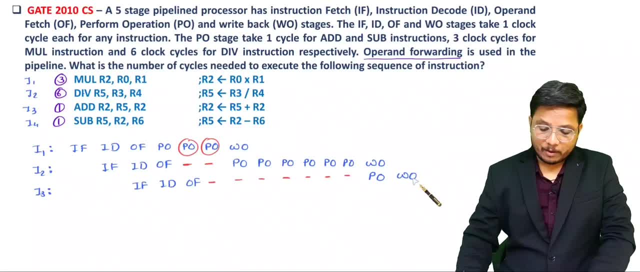 So perform operation can be done here And then write back that we can have right Now. as if you talk About fourth instruction, then in fourth instruction instruction fetch can be done here. Instruction decode can be done here. Operand fetch can be done here. 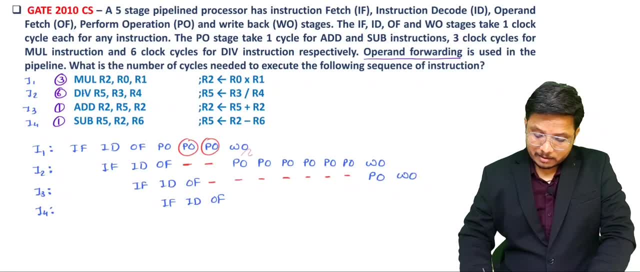 But with perform operation, you see, we are having I2 who is using this ALU, So you'll have to wait. right, You'll have to wait till it is free. Here, you see, I3 is using ALU, So you'll have to wait over here. 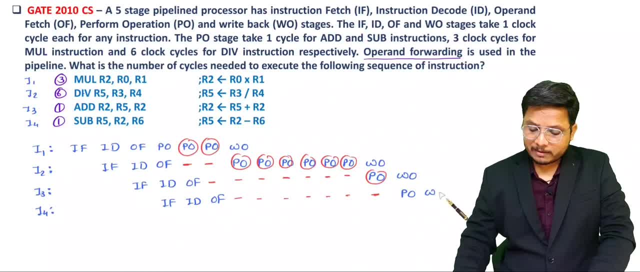 Now over here ALU is free, So we can have perform operation Then And then write back. So if you observe how many cycles that we have used- 1,, 2,, 3,, 4,, 5,, 6,, 7,, 8,, 9,, 10,, 11,- 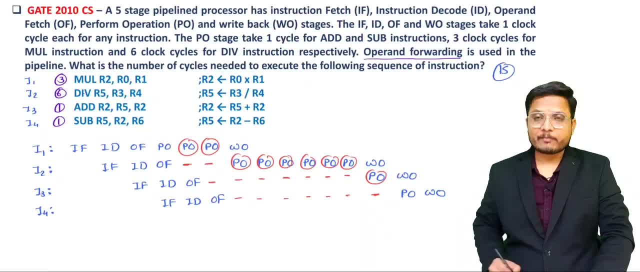 12,, 13,, 14,, 15.. So your answer is 15 over here. But, my dear students, sometimes this method will take too much time. So when you want to solve this in easier way, then how to solve that? 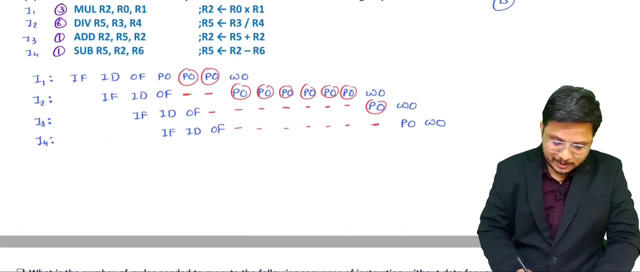 So let me explain you how to do that. So for that, all you need to do is you need to have calculation of cycles. You see How. so cycles will be normal cycles plus hazard cycles. Now, normal cycle calculation that we all know, and plus K, minus one, right. 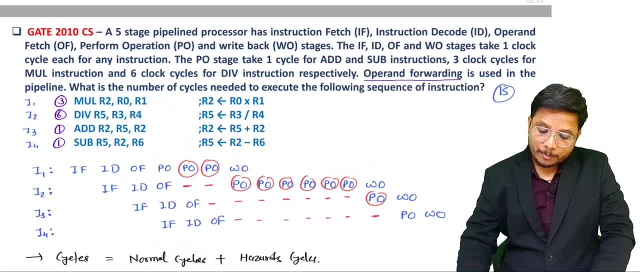 But hazard cycle, how to identify that. So you see, operand forwarding is used, So now you don't need to worry about that data dependency. right After that next question itself, I'll explain you what to do in operand forwarding, right. 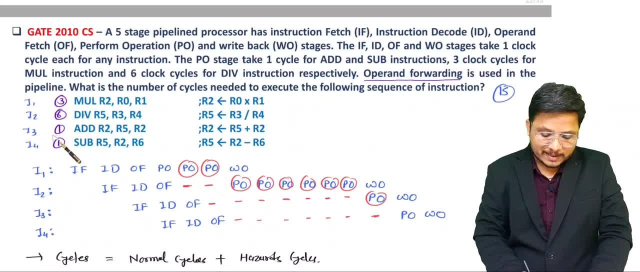 So here you see, with addition, subtraction we are having one cycle With perform operation, but with division and multiplication we need extra cycles. How many extra? with multiplication We need three. Normally we need to have one. So two extra requires for multiplication and division is having six. 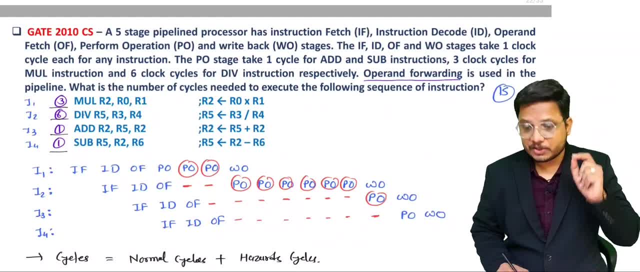 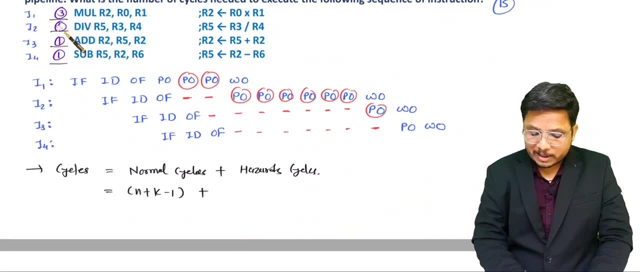 Normally we have one. So five extra that we need to have with division. So you see, hazard cycle for multiplication, How many extra that we need to have to for division, How many we need to have five. So here hazard cycles Are five plus two. now number of instructions here for so any sport, number of stages: five stages are there minus one plus five plus two. so you see what is our answer: four plus five, nine minus one, eight, eight plus seven, fifteen. so your answer that is fifteen. right, you can match it. so that is how simply we can solve question. but now I'm going to add difficulty level more. 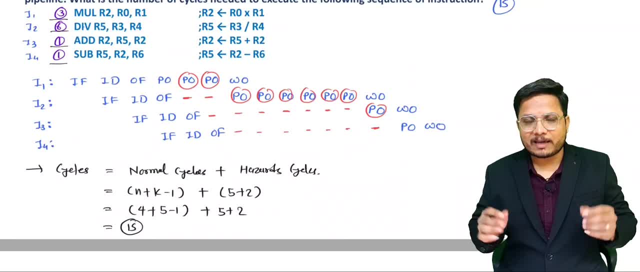 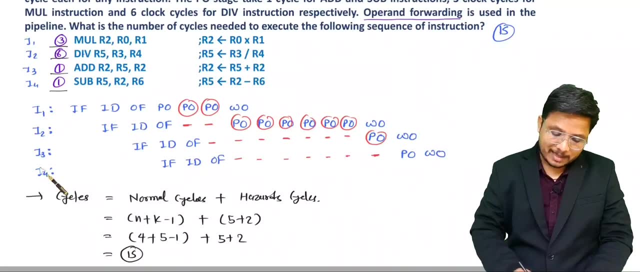 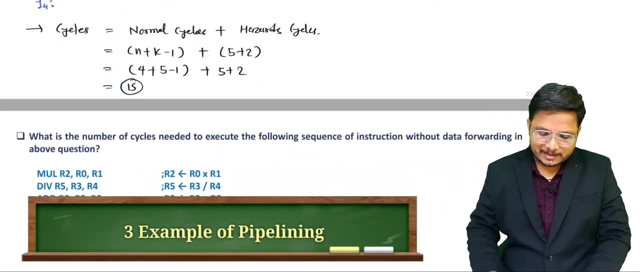 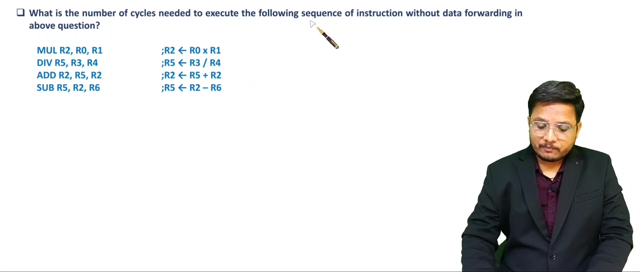 In that we are not given with operand forwarding. so as if it is not given with operand forwarding, then my dear students, this conventional way that we need to follow, but in that also we need to see data dependency. so how to identify data dependency, let us see how. so, question that is given, you see, what is the number of cycles needed to be executed in following instructions, without data forwarding in a book? question. 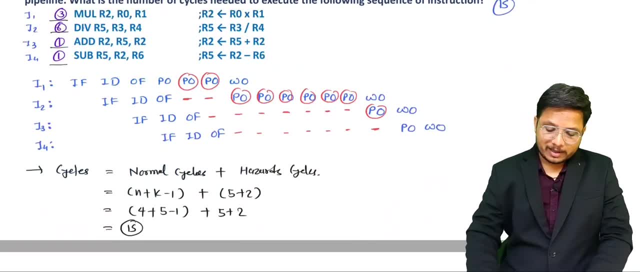 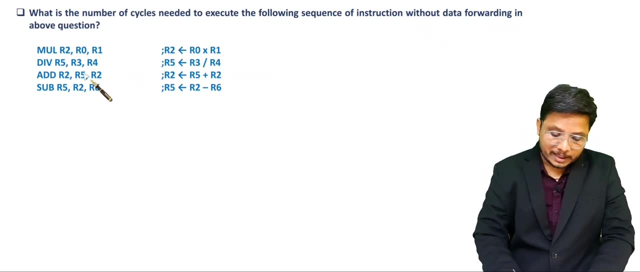 So here, same question is there? Question is same, right, only thing is here we are not having operand forwarding. so as if we don't have operand forwarding, then we need to see how data dependency is there. so how to identify data dependency? so first of all, you should know: these are my input operands, right, these are my input operands and these are my output operands. now you'll have to see whether this output is depending on input of next instruction or not. so you see this. 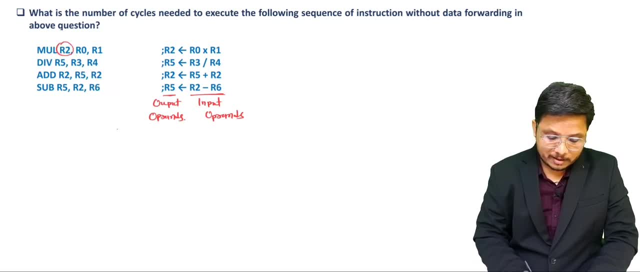 R2 that is not depending on next instruction. right then you'll have to see this R5 is it depending on next instruction? yes, you see, it is depending on over here. this R2 is it depending on next? yes, it is depending on next. so you see, here we are having that dependency, and that dependency that cannot be eliminated, as if you don't have, as if you don't have again, as if you don't have operand forwarding right now. let us try to 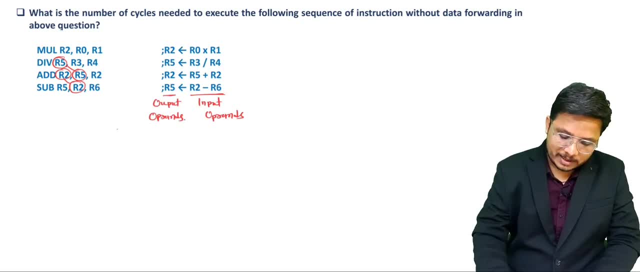 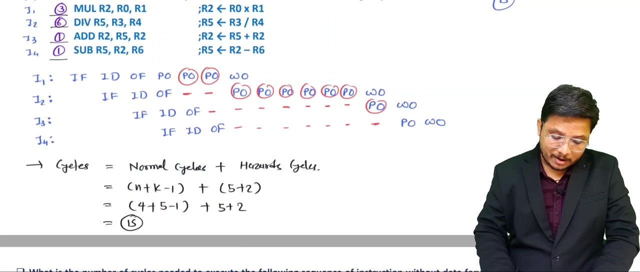 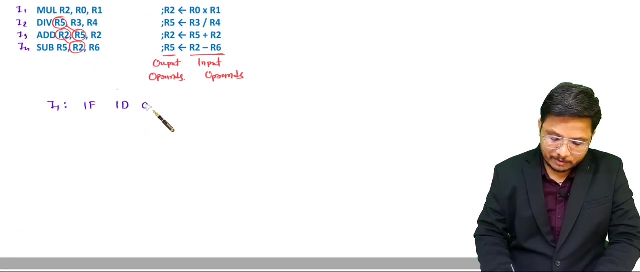 Understand that with respect to timing diagram. so first instruction execution, that will be same. let me write that even I1, I2, I3, I4, right? so let us have I1 over here in timing diagram. so first instruction fetch that we have, then what we have, instruction decode, then operand fetch. let me write instruction decode, then operand fetch, then perform operation for multiplication. how many times you need to have perform operation? 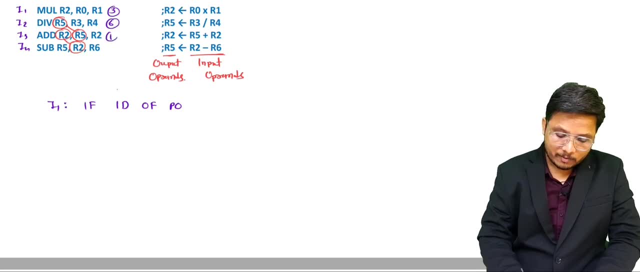 3 times with division, 6 times with add, 1 times with subtract, 1 times. that is given in question right. so first we are performing multiplication, so 3 times we will be having perform operation and then we'll be having write back now second instruction that is not depending on first right. so second, that we can easily make even instruction fetch will happen here, then instruction decode, then operand fetch, you see, then perform operation. that will be having 6 cycles, so perform operation. 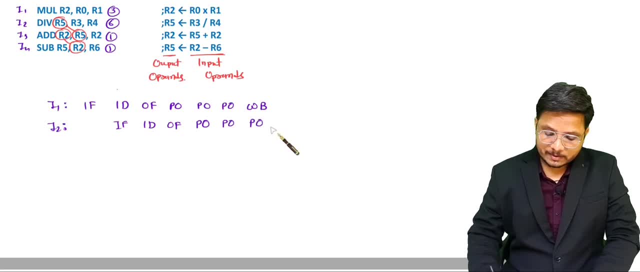 6 times. let me write that 6 times. but here you see, we are having that dependency, right, so you'll have to wait over here. you cannot have perform operation right in hurry, you will be doing mistake here. so operand forwarding doesn't mean like you can overlap ALU, right. you cannot overlap ALU, so here you'll have to wait now, once you wait, once ALU is free, you can provide. 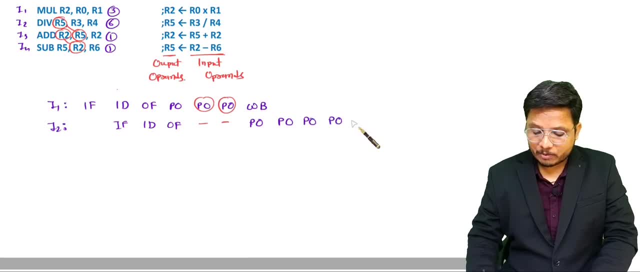 perform operation? how many times? 6 times, you see. I'm providing that 6 times, right? so 1, 2, 3, 4, 5, 6, after that we'll be having write back. now, my dear students, let us have third instruction execution. now, in third instruction, you see, we are having data dependency. RFI is dependent over here. RFI is dependent over here. so here we can have instruction fetch, here we can have instruction decode, but here we cannot have operation. 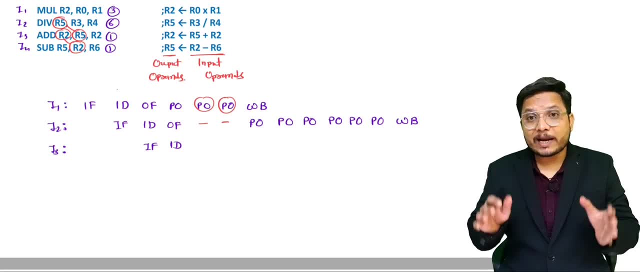 operand fetch. see, for operand fetch you'll have to wait till write back- is happening again for operand fetch. operand fetch means we are taking operands, so you can take operands up to write back. remember this: without write back, you cannot have operand fetch right. so here, my dear students, you see what is happening. first of all, there is dependency. 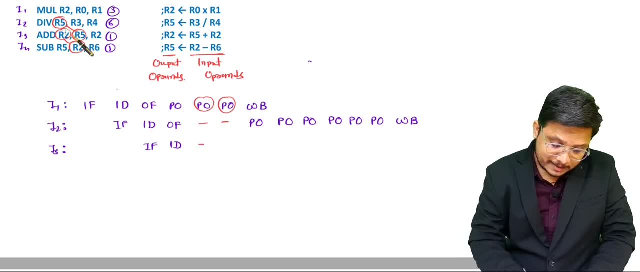 right of that data and this RFI that is there with I2. so here you'll be having RFI, remember this right. so operand fetch that will be having a delay. how much delay? up to this you'll have to wait. once write back is happening, you are free to have operand fetch. then you can have perform operation and for addition, you need to have one perform operation only and then write back. right. 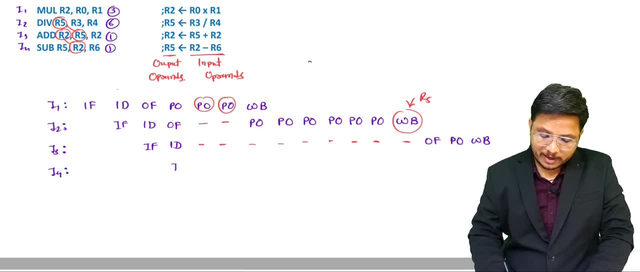 now you'll be executing I4 now in I4. instruction fetch will happen here. instruction decode will happen here. but you see, R2 is depending on output of addition, and output of addition that is happening at this write back only so R2 will come here, right, so you'll have to wait till that is happening. after that only you are allowed to have that operand fetch. so operand fetch that you'll be having over here, then perform operation. 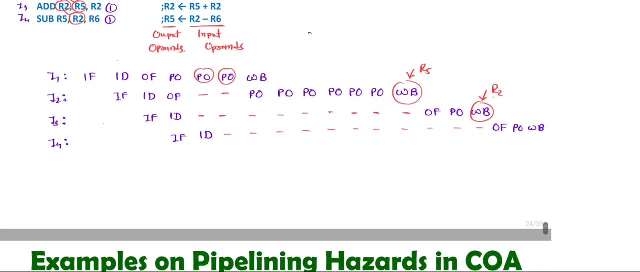 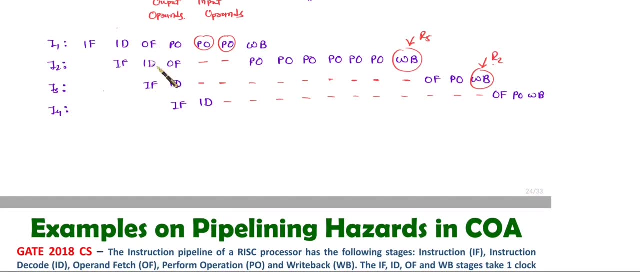 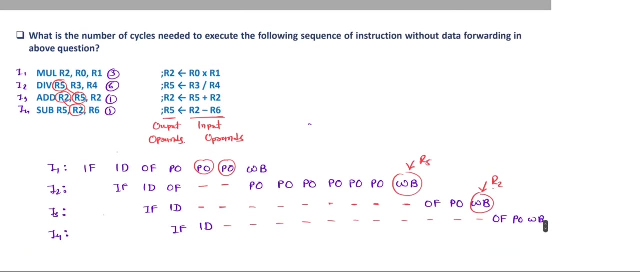 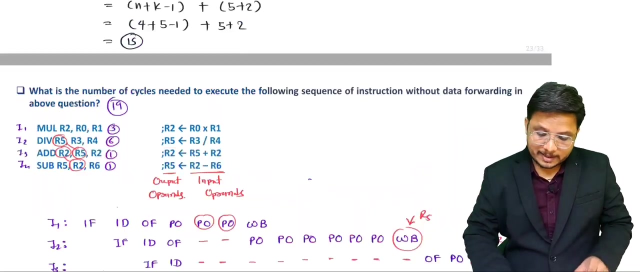 and write back right. so once you have perform operation and write back over here, you can say execution is completed. so how many cycles are there? you see: 1, 2, 3, 4, 5, 6, 7, 8, 9, 10, 11, 12, 13, 14, 15, 16, 17, 18, 19. so with data dependency you will be having 19 cycles, right, and without data dependency, how many cycles that? we have been having? 15 cycles. so because of data dependency, you'll have to add 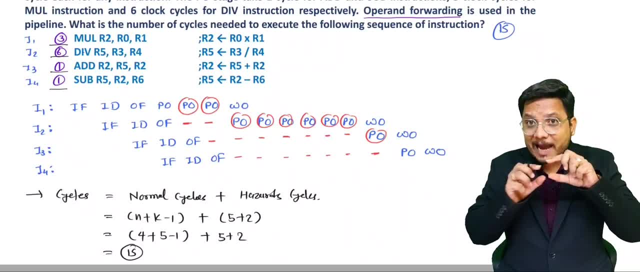 4. another cycles. right, but operand forwarding that word, that is nullifying many things over here. I think now you are having fair enough idea about how to solve problems. still, there will be few more sessions that will be there based on problem solving, of pipelining, that is to improve your fundamentals only right. still, if anything that you would like to share it with me, please note it down in the comment box. I'll be happy to help you. thank you so much for watching this video.